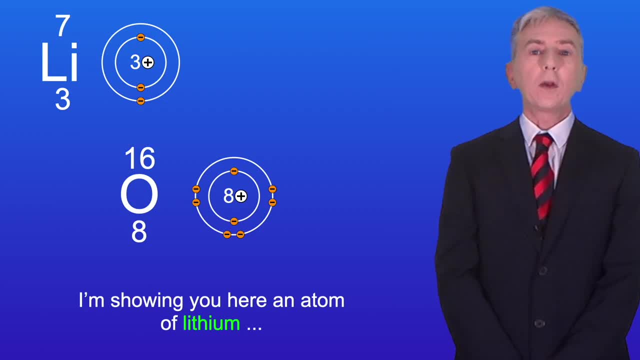 the metals react more rapidly. I'm showing you here an atom of Lithium and an atom of Oxygen. As you can see, Lithium atoms have one outer electron and Oxygen atoms have six outer electrons. When Lithium reacts with oxygen, the outer electron from the Lithium atom moves to the Oxygen atom. 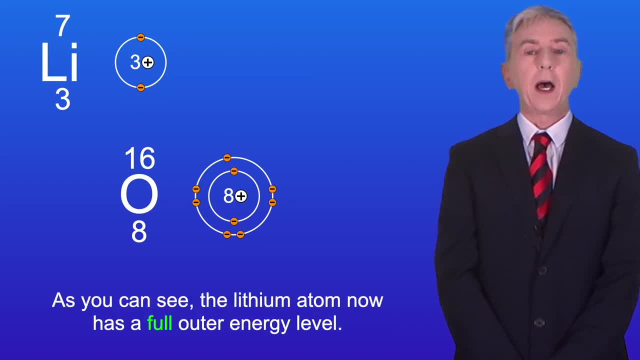 like this. As you can see, the Lithium atom now has a full outer energy level. However, the Oxygen atom does not. Oxygen still requires one more electron. So another Lithium atom now transfers its outer electron to Oxygen like this: Now both Lithium atoms and the Oxygen atom have a full outer energy level At the end. 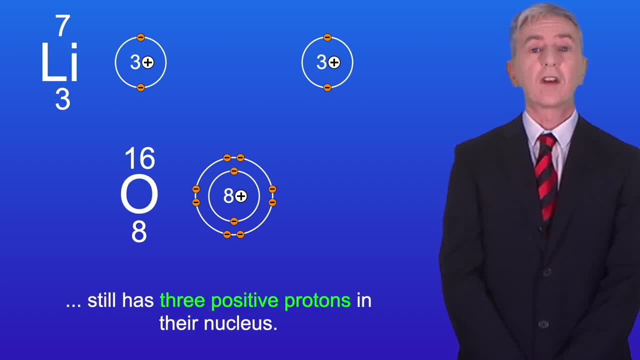 of this reaction, each Lithium atom still has three positive protons in their nucleus. However, they only have two negative electrons, so these are now Lithium ions with a positive one charge. The Oxygen atom still has eight positive protons in its nucleus, However. 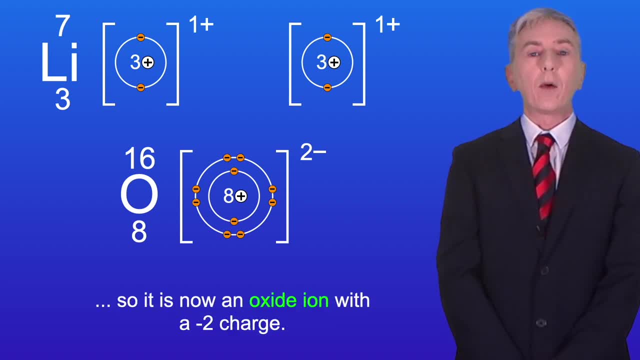 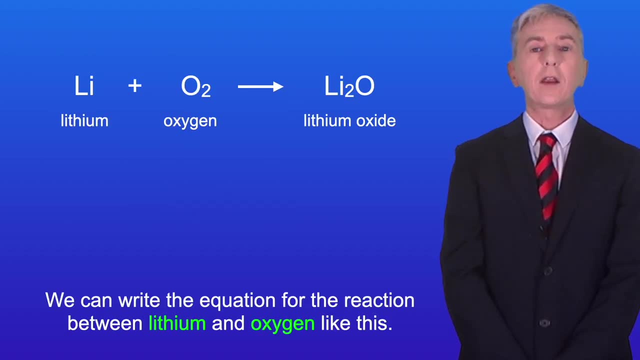 Oxygen now has ten negative electrons, so it's now an Oxide ion with a negative two charge. We can write the equation for the reaction between Lithium and Oxygen like this: Remember that Oxygen molecules contain two Oxygen atoms. This means that we have to balance the equation. 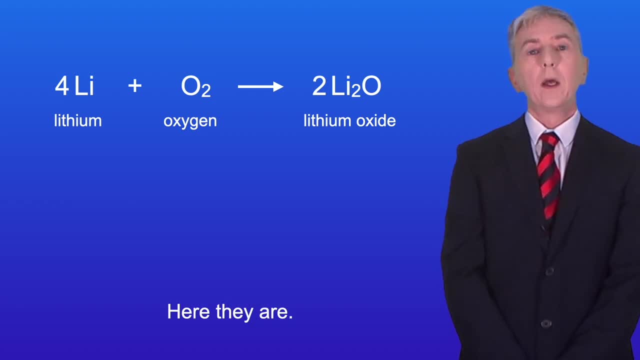 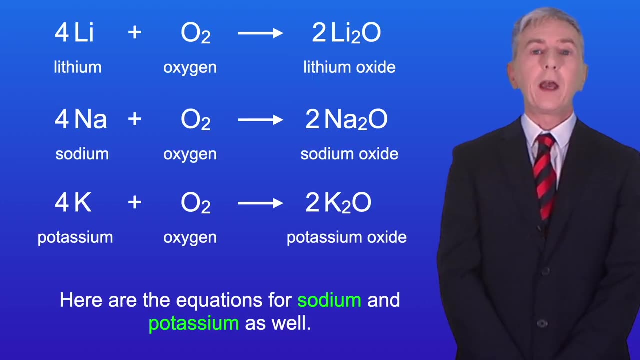 by inserting large numbers, and here they are. We can write equivalent equations for other Group 1 metals simply by changing the symbol for the metal. So here are the equations for Sodium and Potassium as well. Now, because all of the Group 1 metals have one outer electron, they all react with Oxygen. 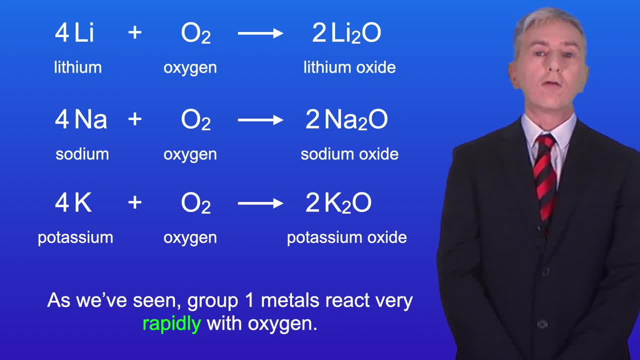 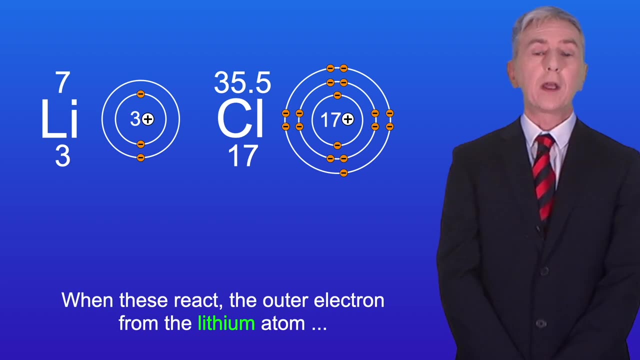 in the same way. So, as we've seen, Group 1 metals react very rapidly with Oxygen. Group 1 metals also react rapidly with Chlorine, which is in Group 7.. This shows a Lithium atom and a Chlorine atom. When these react, the outer electron from the Lithium atom moves onto the Chlorine. 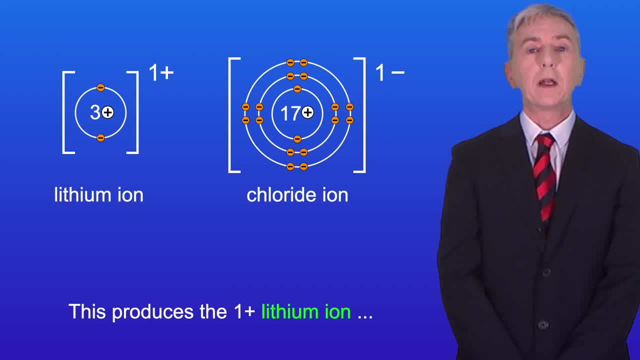 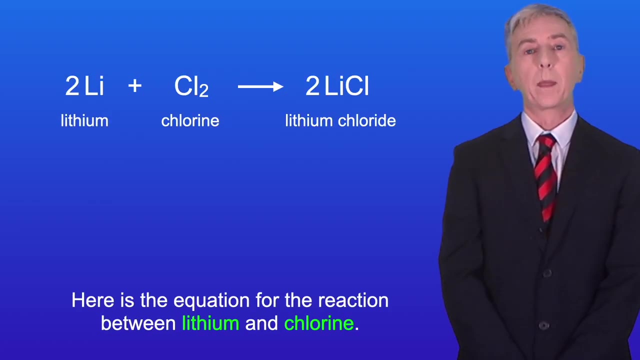 atom like this. This produces the 1-positive lithium ion and the 1-negative chloride ion. Both of these ions now have a full outer energy level and we've made the compound lithium-chloride. Here's the equation for the reaction between lithium and chlorine.